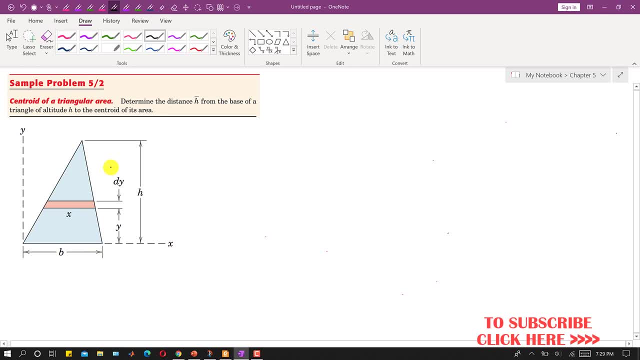 triangular area and we are required to find the centroid of this right. so, to determine the centroid of this rectangular area, what we will do is that we will select a differential strip right, this differential area right, since we are required to determine the distance H from the base of a triangle. 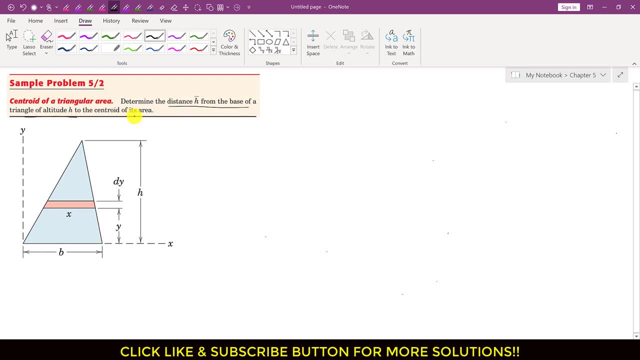 of altitude H to the centroid, to the centroid of its area, right. so we are required to find the distance from the base of this triangle, right. so this means that select us, the differential element that is parallel to the x-axis is right and that differential element should be like this, right. we should divide this. 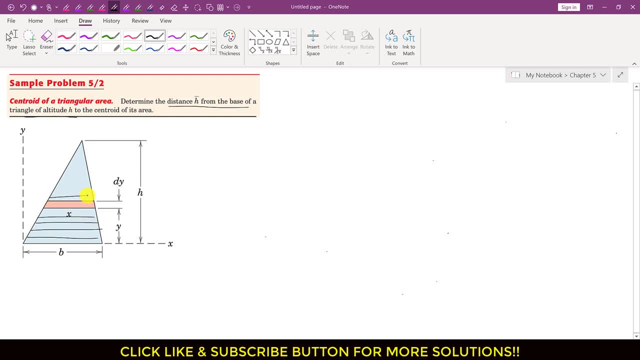 triangular area in this horizontal like strips right, and these strips should move along the y-axis is right, since we are required to find the centroid along the y-axis is right. so to find that distance from the base. what we will do is that we will select this differential area right and the this. 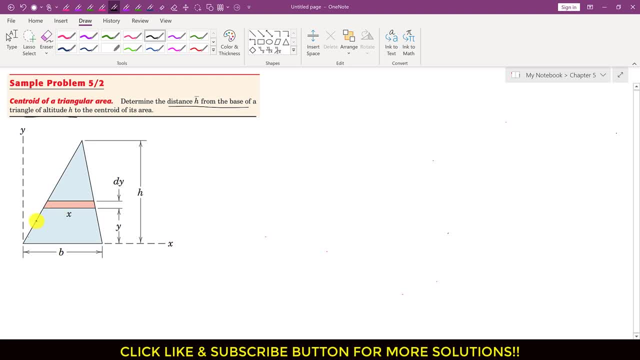 this length is equal to X right, since it will vary along the y-axis, is right. this X the, this length of this differential area is a function of Y right. so we can say that X is a function of Y right. it varies along the Y coordinate right. 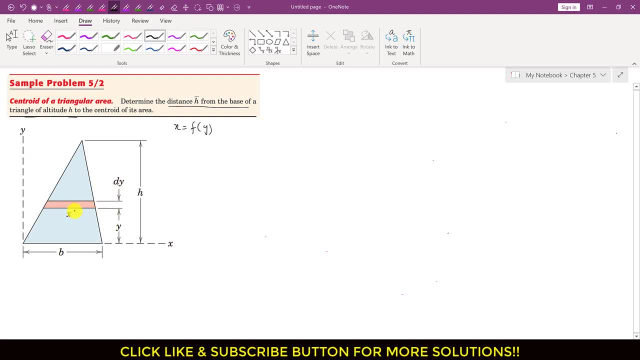 along the y-axis is right. and let's say that this differential element is at a distance of Y from the base, right from the base or from the x-axis, is right. so this is that Y coordinate and the thickness of, or we can say that the width of this differential area is dy, right, so this is that dy, and 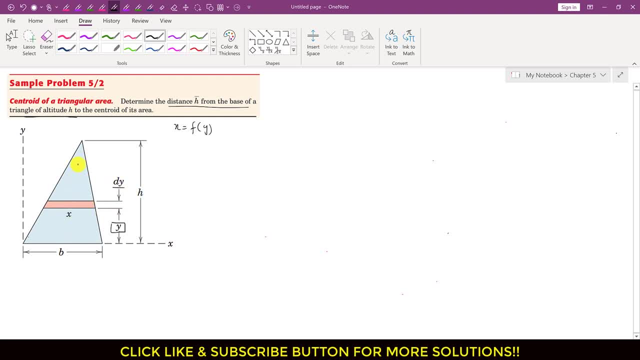 the total height of this triangular area, or the altitude of this triangular area is equal to H, right? so now, since we are finding the centroid of an area of a triangular area, so we will apply a the equation for the centroid equation for areas, right? so we will write that we. 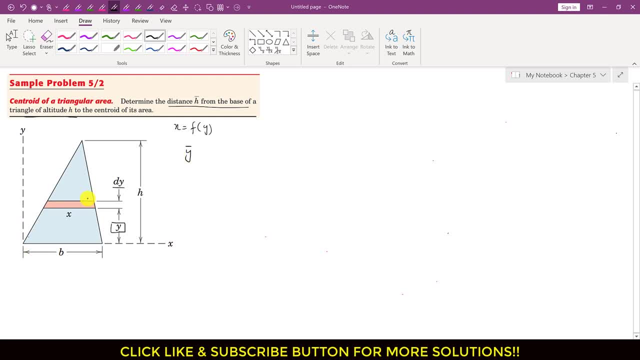 since we want to find the distance along the y-axis right. so we will use this equation, that is, y bar and this will be area right. or we can say that it will be y da and this will be equal to integral y C and this da right and this integral. 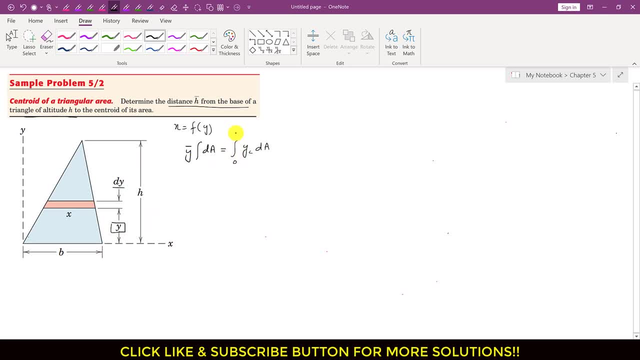 will be from 0 to H, right? so I will write that this is 0 to H, and similarly, we will have 0 to H here. let's say that the centroid of this differential area is somewhere here, right? and this since this is a differential area. so this dy. 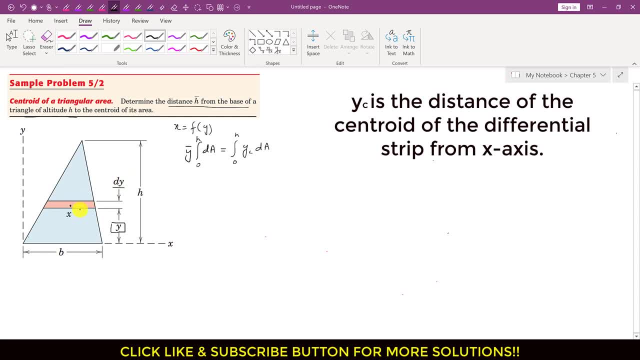 is very small, as we know, right. so let's say that the centroid of this differential element that is at a distance of y right, so this means that we can say that y C is equal to y right. so y C is equal to y right, this, this, let's say that this is: 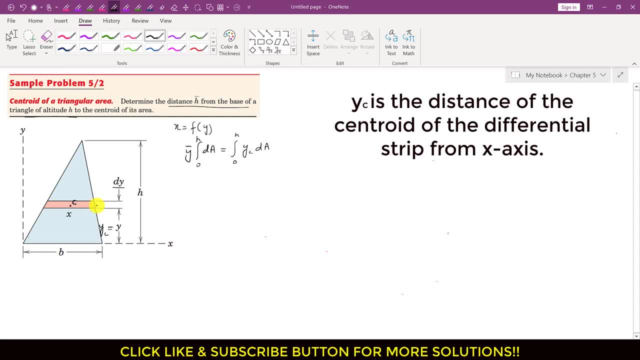 the centroid of this differential area, right, this small c. so then we can say that y, C equals to y and we can write da equals to da. is the area of this differential strip, right? so we can say that this will be x times dy. right, so we can write: this is x. 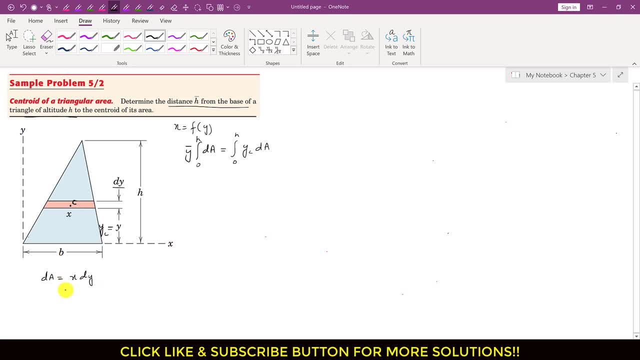 dy right. and if we want to find only this integral right, this d a from 0 to h is, we know that the area of a triangular geometry is half base into h right. so we know this integral right, so we can write that this y bar is. 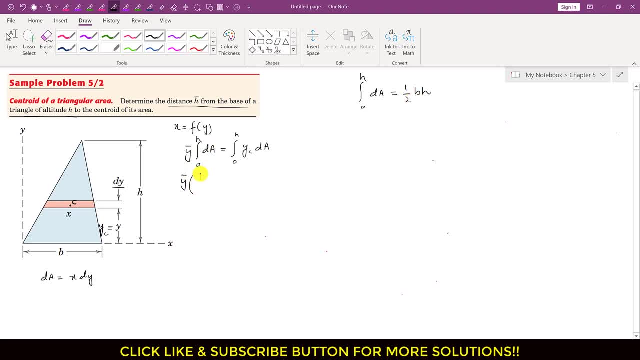 we can replace this by this right, so this is half base is b right, so base is b into h right. and then this is from 0 to h and y c right, so y c is equal to y right. so we can add: this is y and d, a is x, d y. 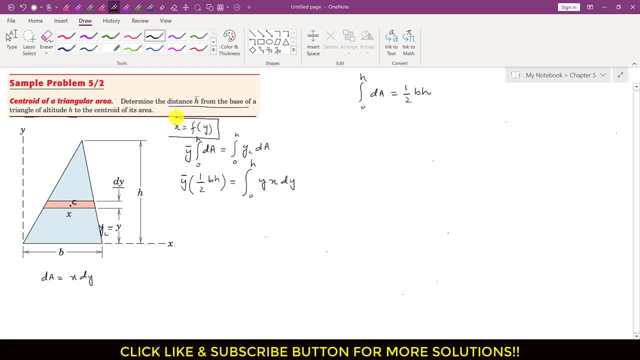 right. so, as i told you people, that x is a function of y right, so we have to find that x has a function of y, since the integral of y is y right. so we have to find that x is a function of y. integration is with respect to y right, so we cannot integrate it until and unless we have the 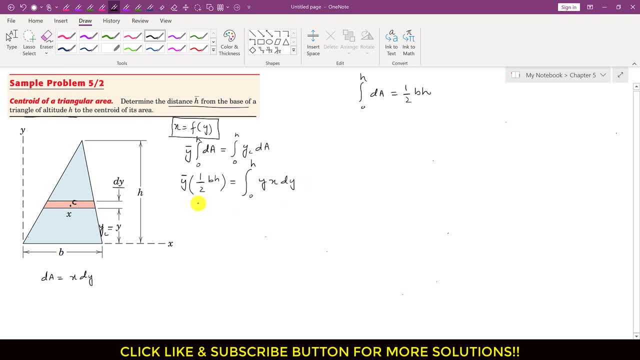 x as a function of y, right. so now, as we can see that, if i consider this triangle, let me write that if let's say that here we have one, two, this point, this point is: let's say two and this, let's say one unless it's three, and let's say that we have, let's say this is a four and let's say this is five. 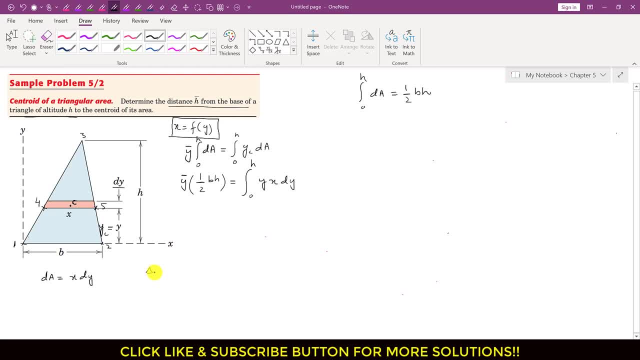 right. so now our triangle one, two, three and triangle three, triangle four, five, three. they are similar triangles, right, one, we have one, two, three triangle, this large triangle, this whole triangle, and then we have this four, five, three triangle right, for both of these are similar triangles. so we can find this x by using the properties of similar triangles. right, let's say: 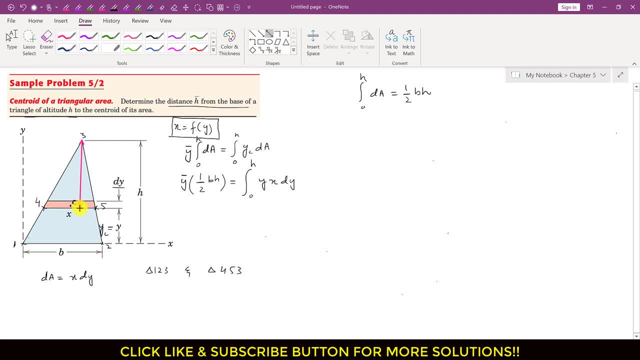 that this is the height of this. yeah, yeah, small triangle, right, this 453 triangle, right? so what will be this length? so this length will be H minus Y, right? so the height of this 453 triangle, the altitude of this 453 triangle, is H minus Y. right, so we can take the ratios of the. 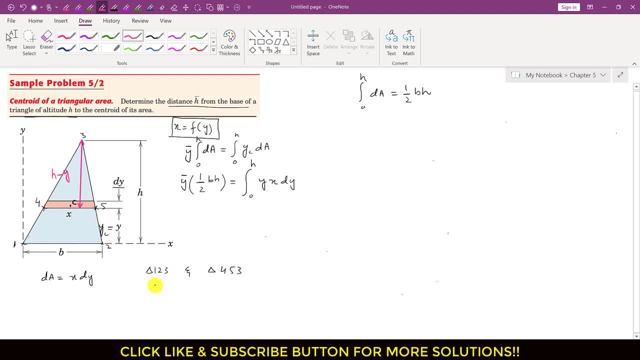 base and the altitude right. so I can write: X divided by H minus Y, this will be equal to B right. this B divided by H, the altitude of the large triangle. this is the altitude of the small triangle right and this is the base of the small triangle. so this ratio will be equal right. so from this we can read that X is: 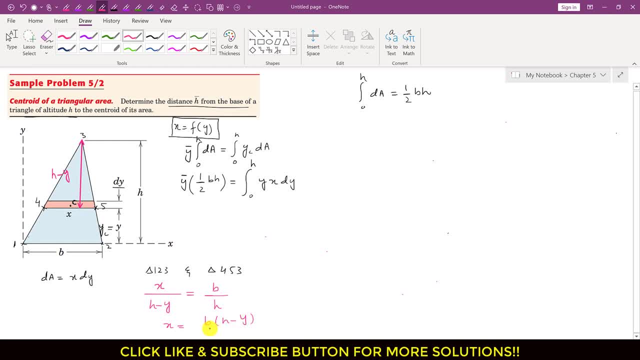 equal to B into H minus básicamente Bx divided by h, right? so this is the x as a function of y. so now we can, we can, we can find this integral right. so let me write that this integral, let me first find this integral- only right. so this: 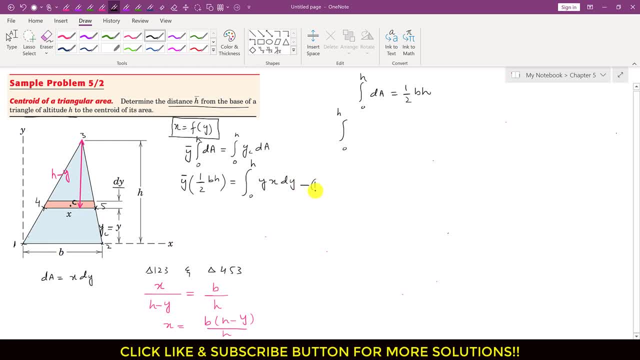 is from 0 to h. let's say this is equation 1, right? so this is y into x, into dy, so we can write that y, now x. is this right? so we can replace x by that function, right? so this b into h minus y divided by. 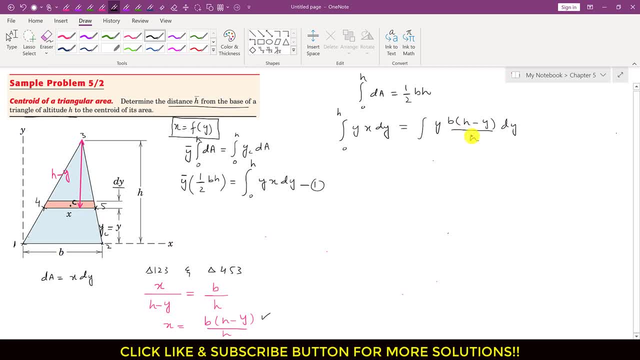 h and this is dy right. so b and h are constants, now right, and this is from 0 to h. so now, if i take b divided by h- common right, so we have this b divided by h, this is from 0 to h, so we can. 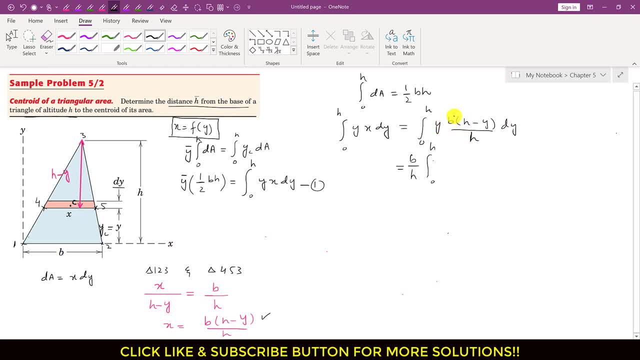 multiply this, right. sorry, we can multiply this y with h right. b and h are common, right? so this will be hy minus y square dy, right? or we can split it right. we can write it like this: so b divided by h, this will be from 0 to h hy dy minus from 0 to h y square dy. 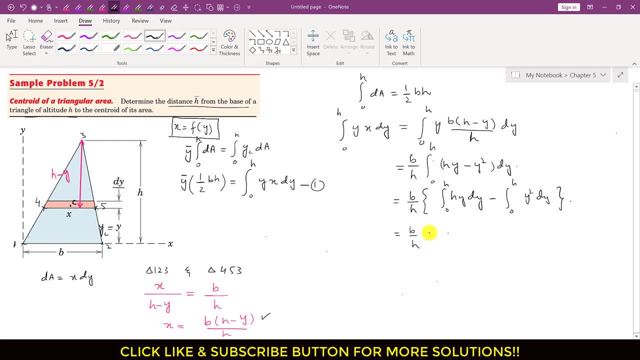 right. this is b divided by h. so the integration of this will be: we can take h common from this integral as well. so this will be h y square divided by 2, from 0 to h minus, and this will be y cube divided by 3, and this is from 0 to h right. so this is b divided by h. and if you put 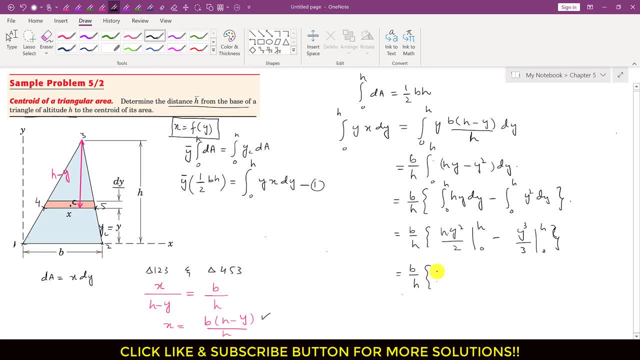 these limits. so then this will be h into h square divided by 2 right, so this will be h cube divided by 2 minus 0 right. and then this is minus, and this will be h cube divided by 3, so 1 by 2 minus 1 by 3, so 1 by 2 minus 1 by 3. so this: 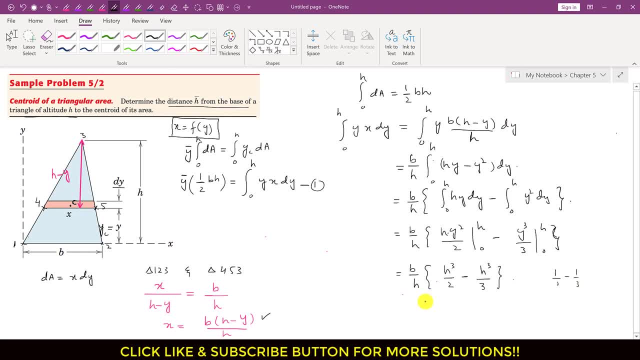 is uh 1 by 6, right? so from this we can write that this is b divided by h and from this we get h cube by 6, right? so then this h will cancel out. so then this integral is equal to b- h square divided by 6. 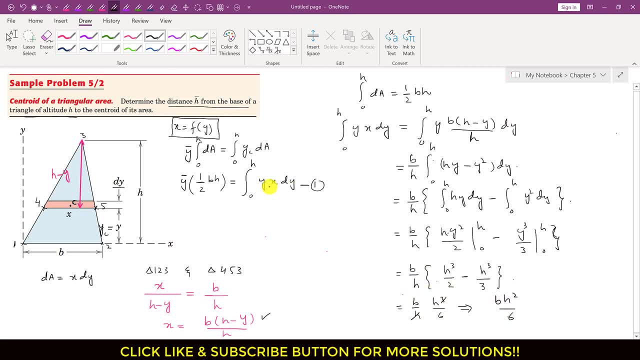 right, so now we can put this integral in this equation: 1, right, so we have this equation: this is y bar is 1 divided by 2, b, h and this is b h square divided by 6. right, so b will cancel out. we can cancel out this b. this 1 h will be cancelled out and this will be cancelled out. 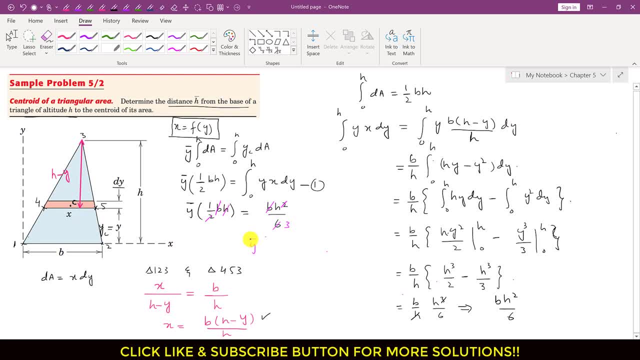 and we will have 3 right. so this means that y bar equals to h divided by 3 right. so this means that the centroid of this triangular area is at a distance of h divided by 3 from the base of this triangle right. so let's say that somewhere here is that that c point. 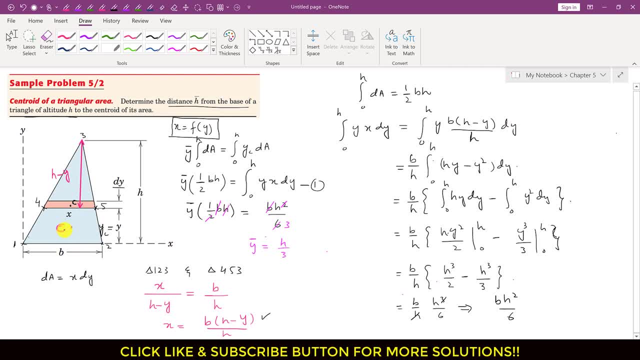 right, right, this is that capital c, this is the centroid of this whole area, right? so the y coordinate of this centroid is h divided by 3. so now, what does this means? that if, if this h is, let's say, 9 meters, right, so then this centroid will be at a distance of 9 divided by 3. 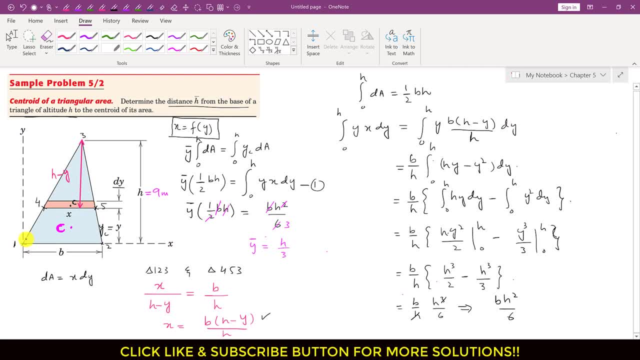 so at a distance of 3 meters, uh, from the x axis, right? so this means that in that case, this distance will be 3 meters. now, if we rotate this triangular area and have some other orientation, right, let's say that this is a, this is our, that one, three side, right. so this is one, three, two. right now we are. 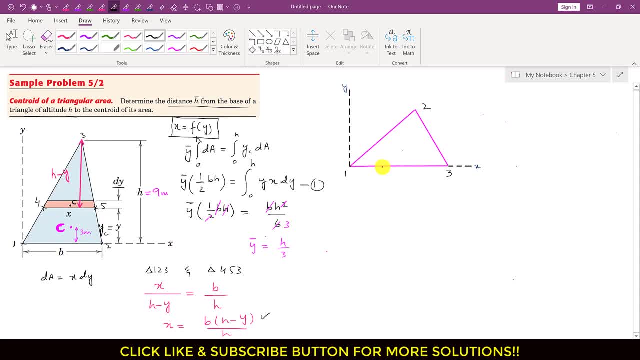 considering that this one three side as a base of this triangle. so let's say that the length of this one three side is, let's say, a right, and let's say that now this height is, let's say, h a. let me write: this height, this altitude, is h a. so now again, if we repeat that same procedure and if we consider that this: 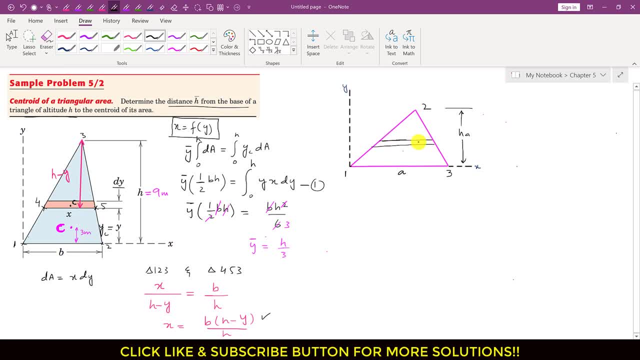 as a differential element, this differential strip as a differential area. so then we will have a that y bar equals to h, a divided by 3. and similarly, if, if i rotate this and if i place this triangle in some other orientation, if we consider this two, three as the base of this triangle, so then we will have: 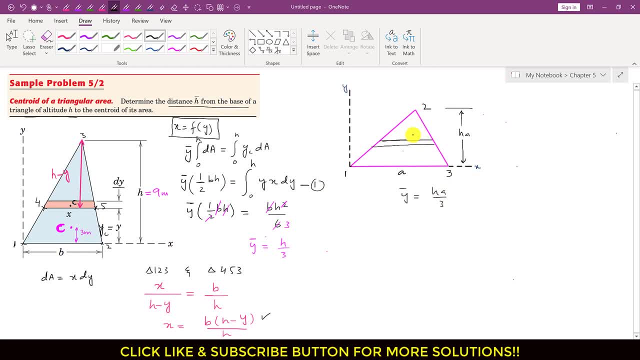 again, uh, the altitude, in that case divided by three right. so this means that the centroid of a triangular area always lies at the intersection of the of the medians right. so what are what is median? so median of a triangle is the line from this vertex to the